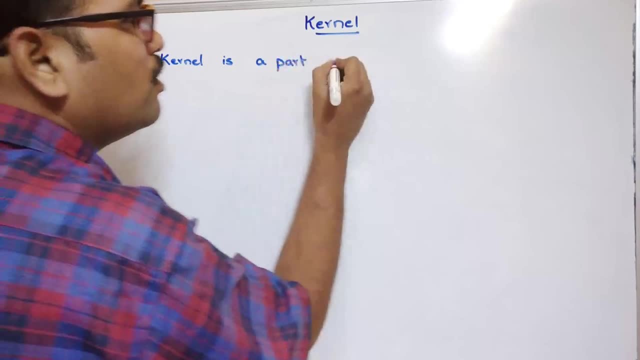 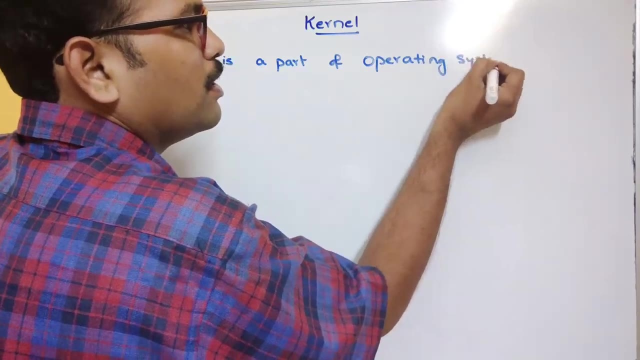 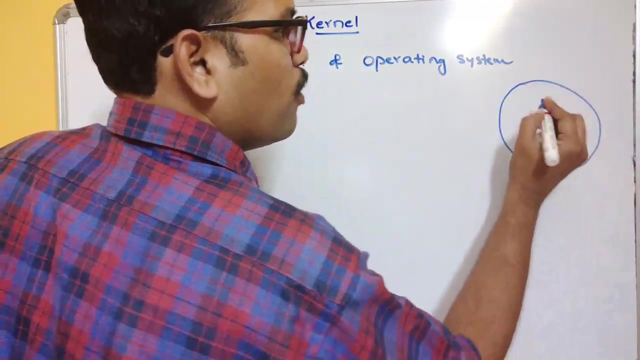 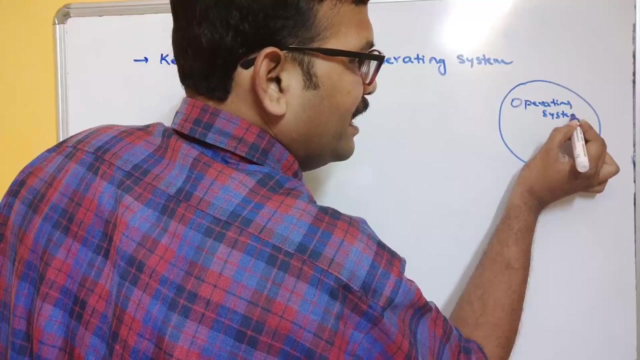 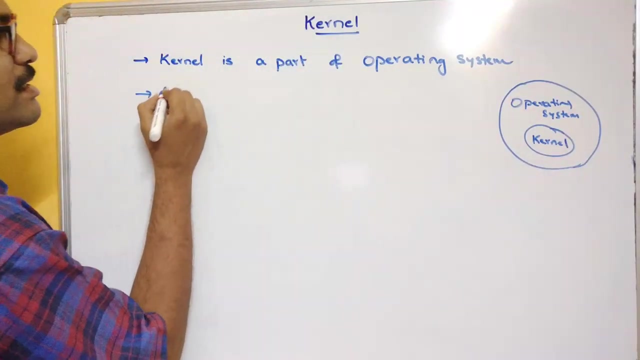 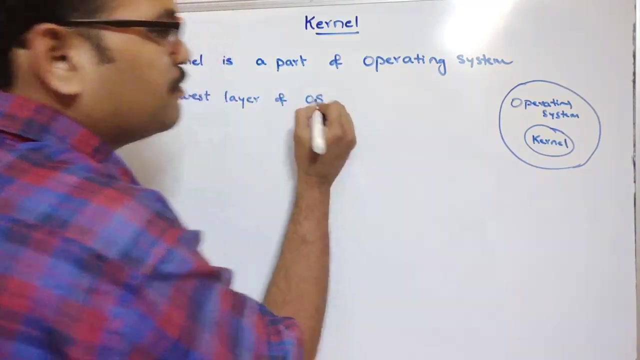 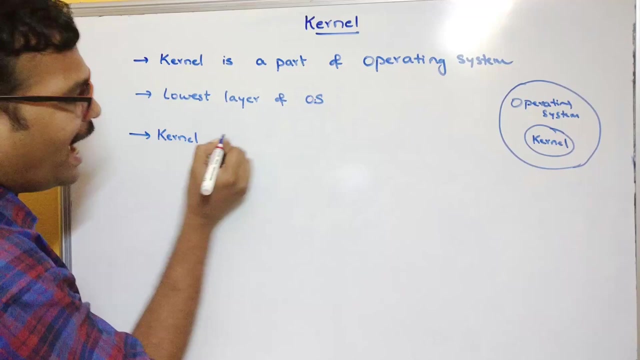 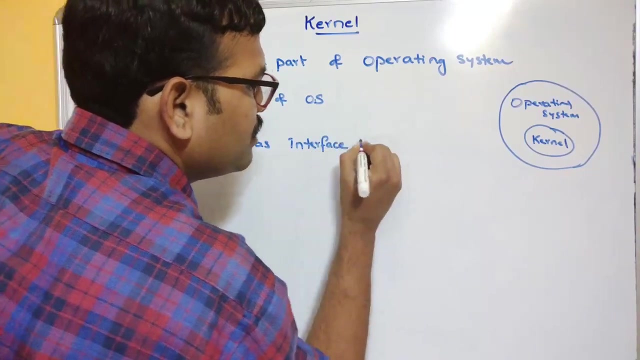 a path of operating system, A path of operating system. So this is an operating system, And in this there is one more layer that is called kernel. A kernel is lowest layer of operating system, Lowest layer of operating system, And also this kernel will act as interface, interface between hardware and hardware. So this is a 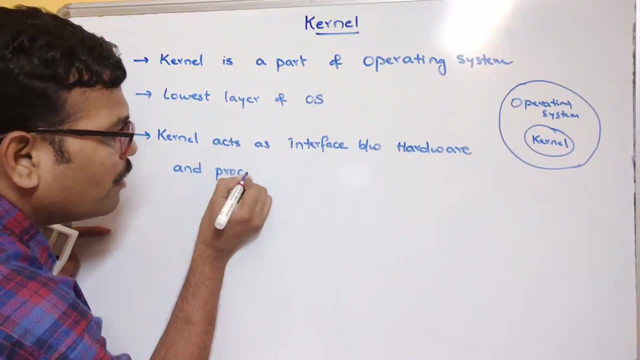 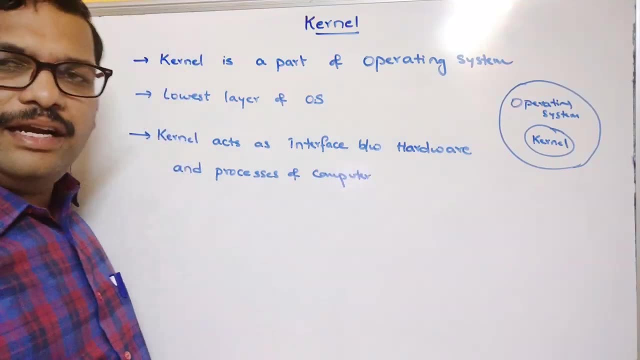 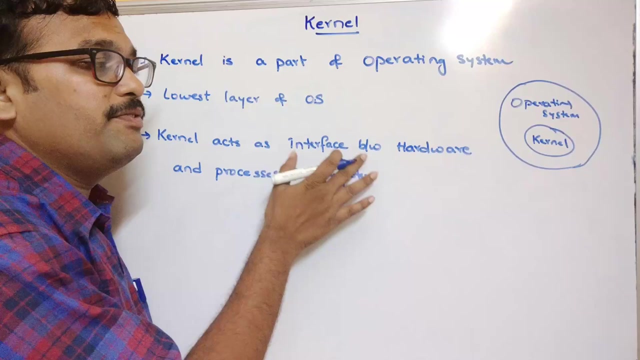 path of operating system And processes of a computer. So we can simply say the software applications, right? So whatever the applications we are executing in our computer, so the kernel will act as the interface between the hardware and the applications of a computer, right? 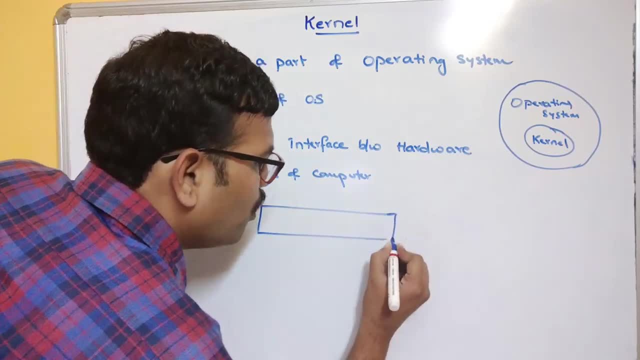 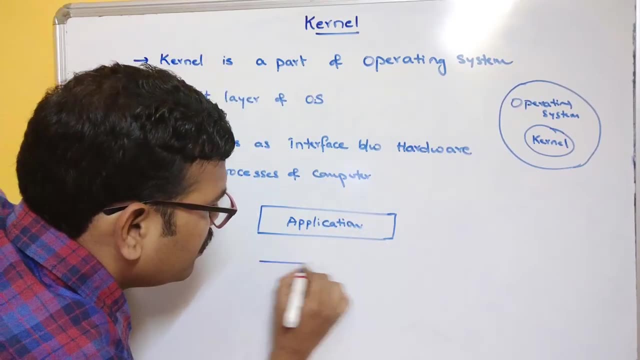 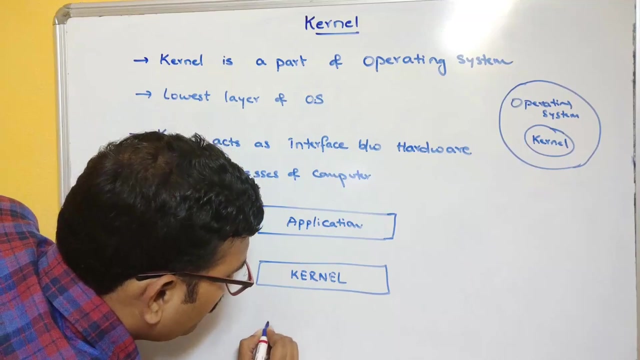 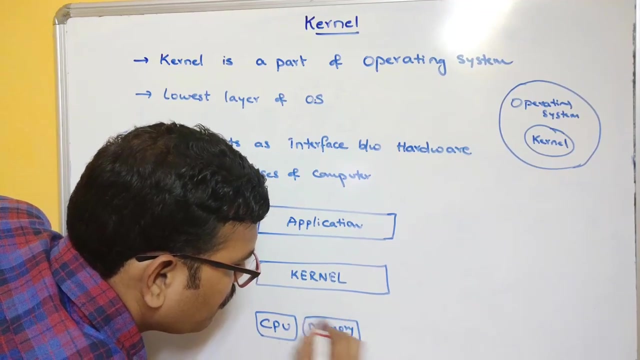 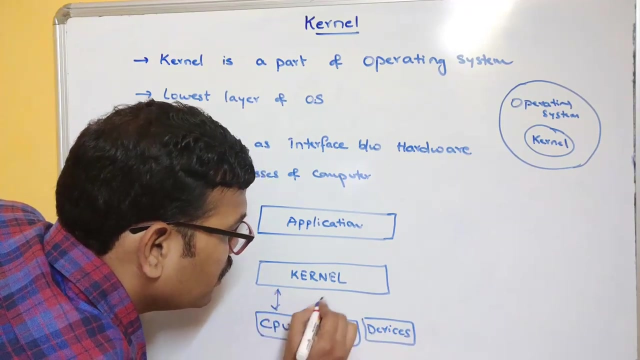 See, let us assume this is an applications. All these are the applications, So it will be unnecessary for us to base it on the hardware application. So the kernel is going to act as the interface between the application software applications, right, The application software. So the kernel will act, act as a 좀 little flight, and they will 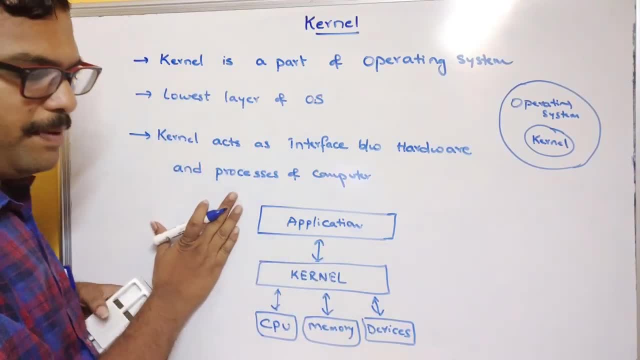 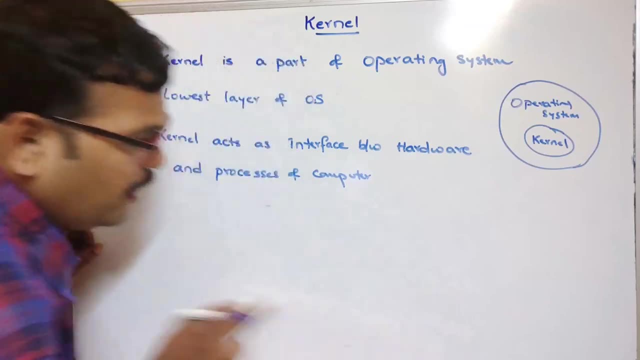 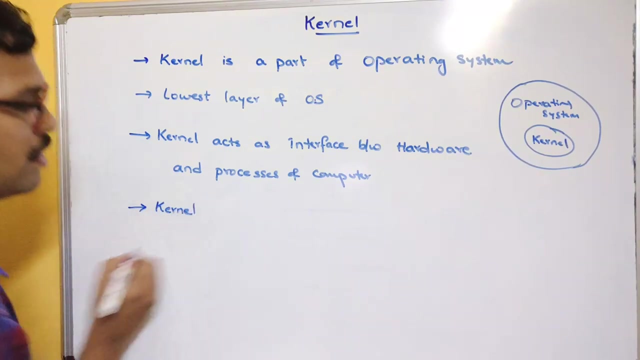 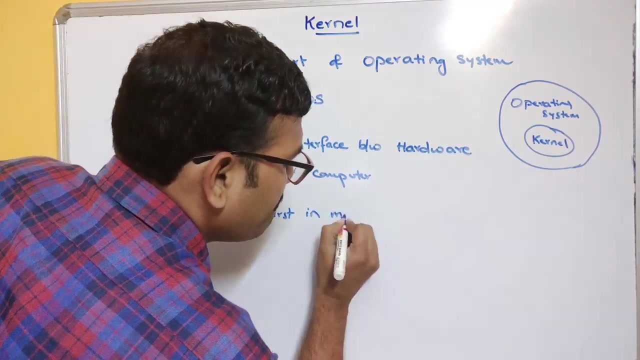 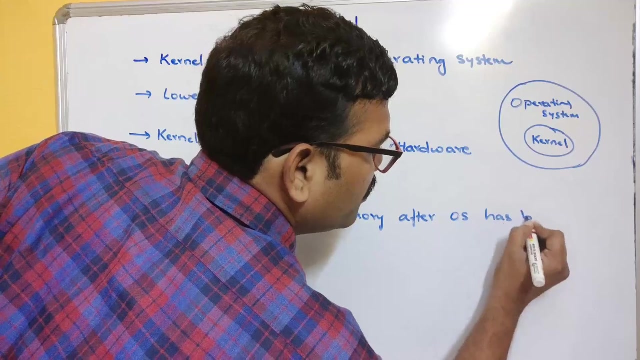 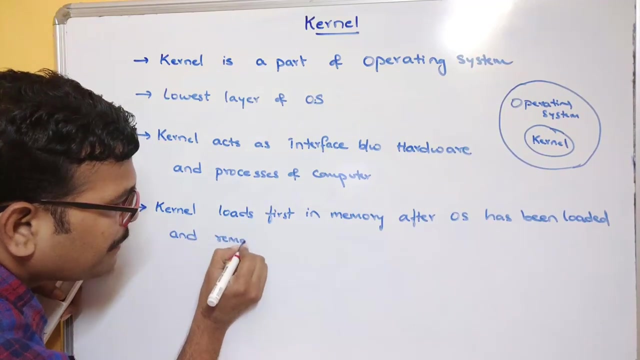 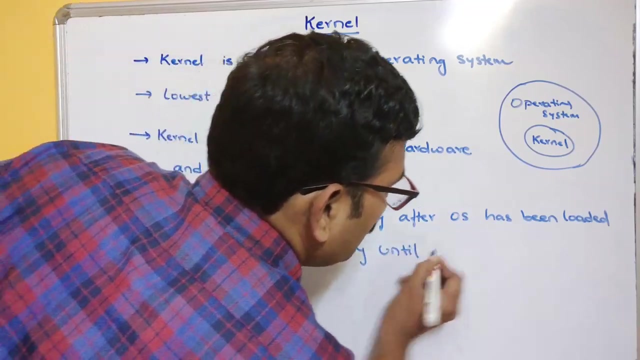 start like this: The kernel will go back to our computer So when it engaged a kernelitating these applications and the hardware. so this is a hardware right and here the kernel loads first in memory after voice has been loaded and remains in memory until operating system is shut down. so we know that. so 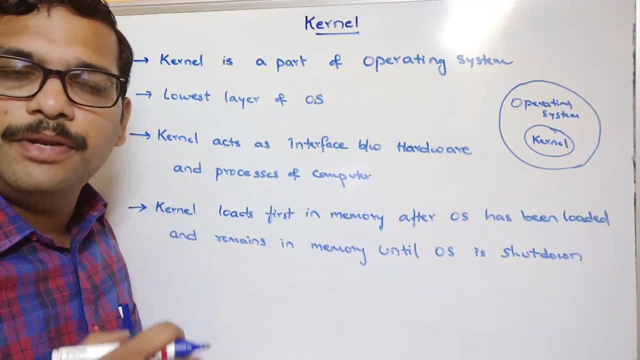 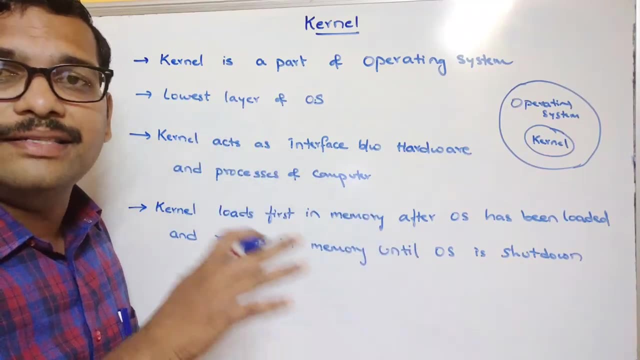 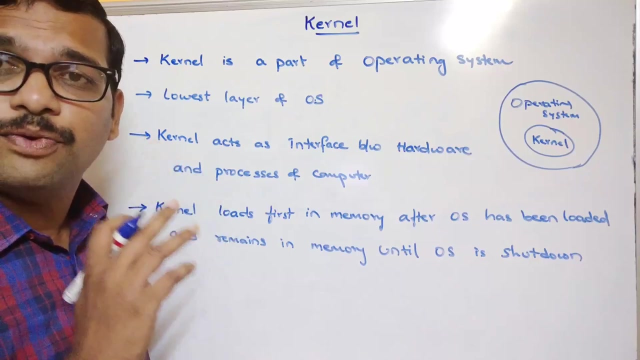 once you switch on, switch on the system- the operating system will be loaded and immediately the kernel will load first in the memory and it will resides in the memory itself until the system gets shut down. so what are the functions provided by this kernel, what this kernel actually do? 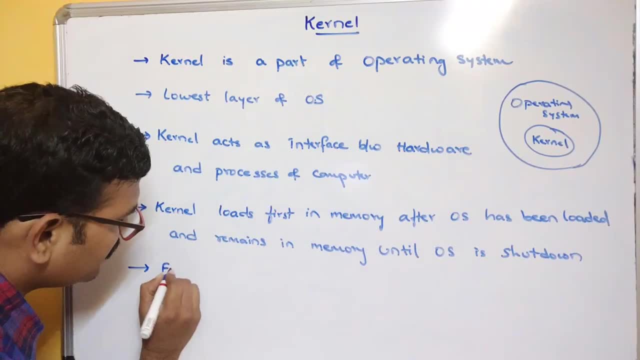 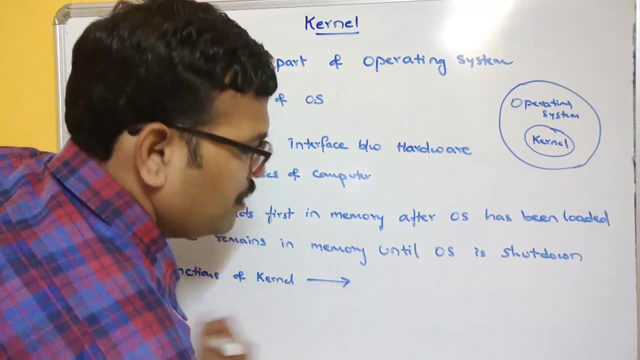 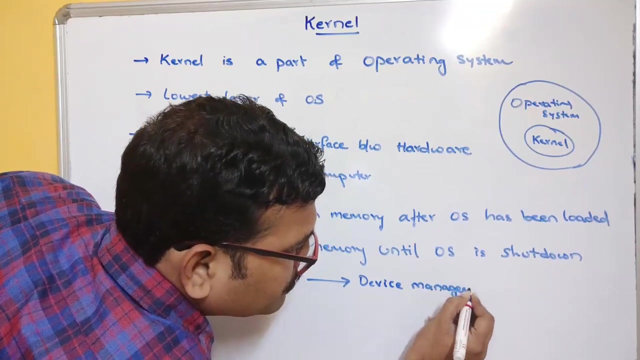 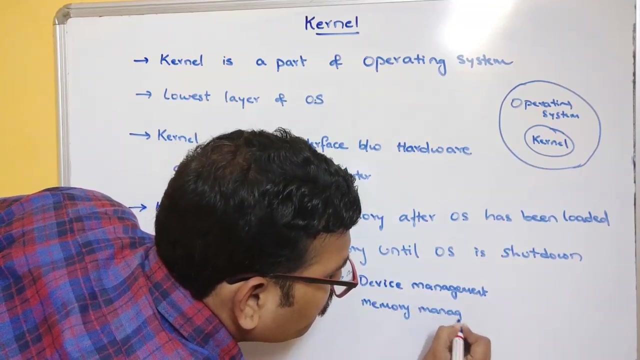 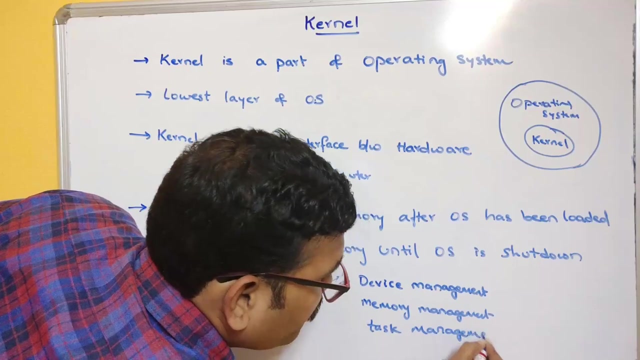 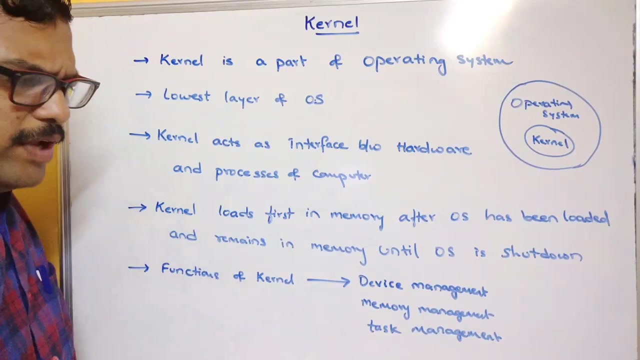 so the kernel? the functions of a kernel are device management, allocating the devices, memory management, task management. so these are all the different functions provided by the kernel itself. right? so we have discussed about all these things in the previous sessions. what is the device management, what is the memory management and what? 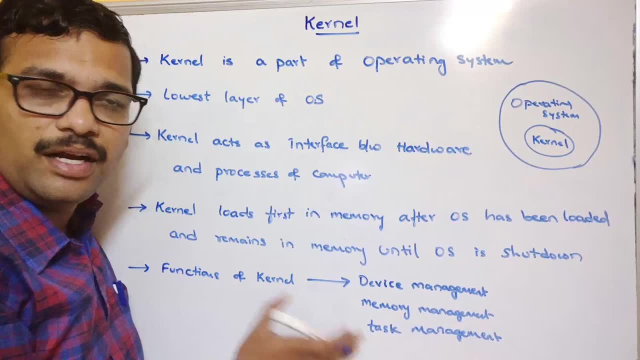 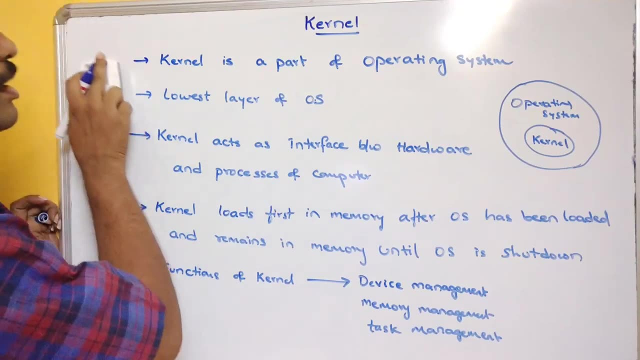 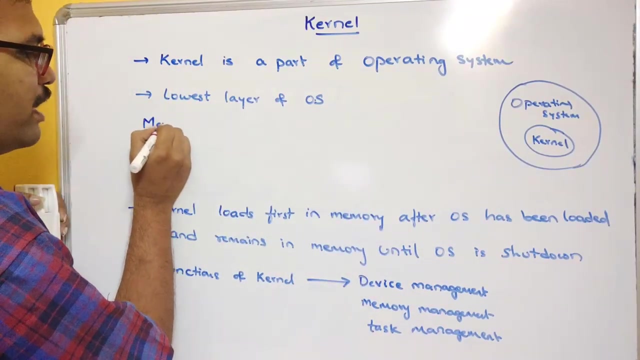 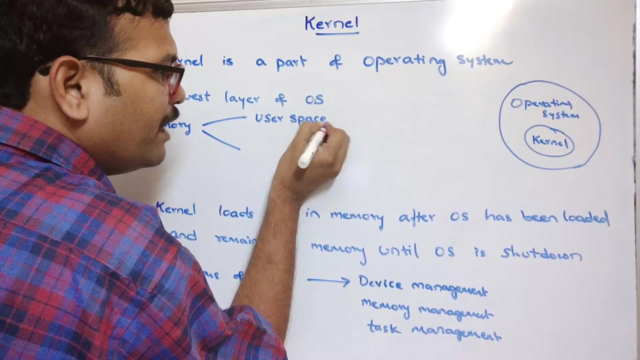 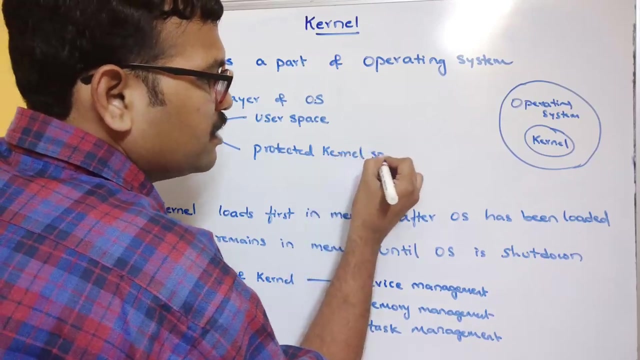 is the task management, everything we have discussed in the previous sessions. right, so? so these are the functions provided by the kernel itself, and here the memory is divided into two types. one is a user space and another one is a protected kernel space. protected kernel space, so in the user. 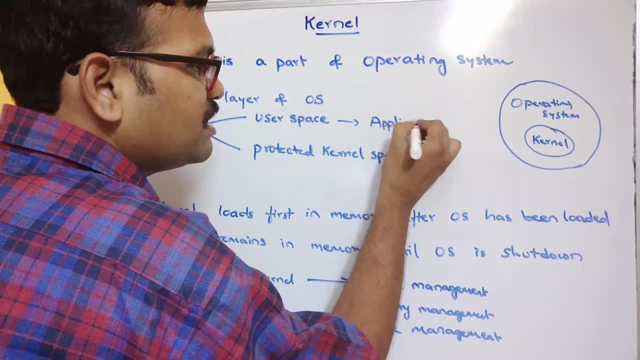 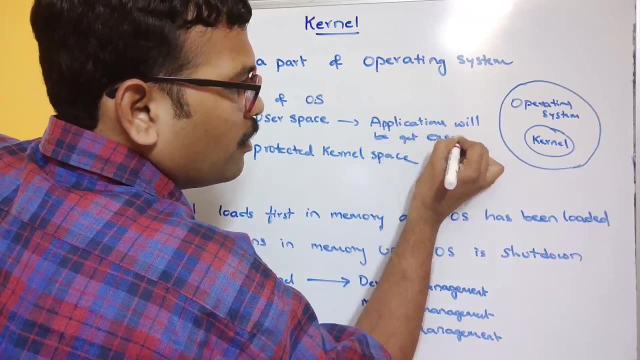 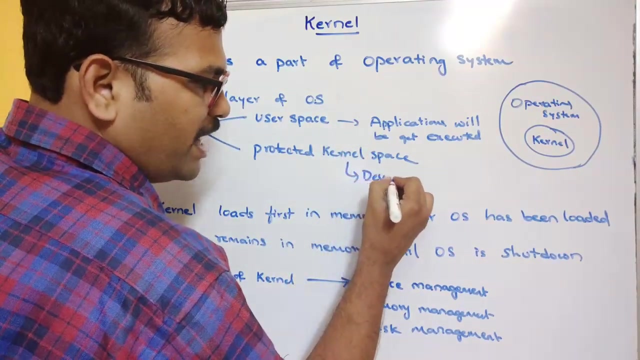 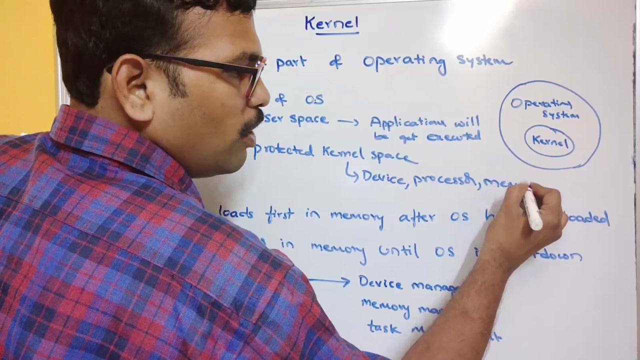 space, all the applications, all the applications will be get executed, so in the protected kernel space. so all these services will be done. that means the device management, okay, processor management or task management or memory management. so all things will be done in here itself. so these are not visible to 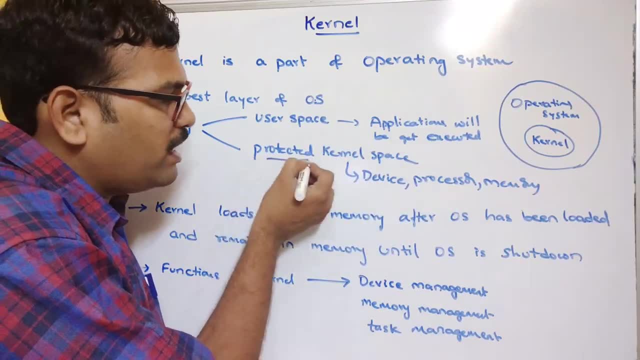 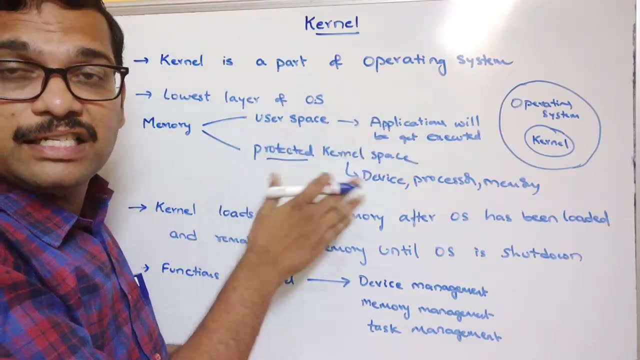 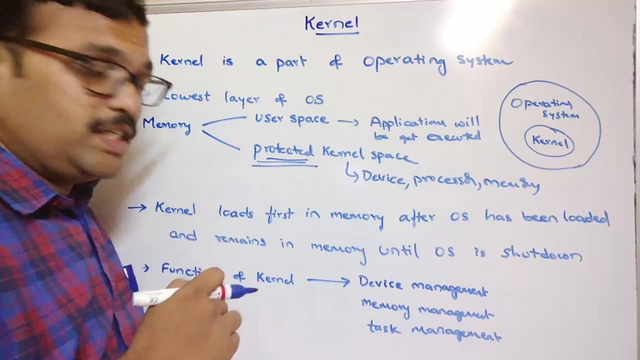 the user and here the name itself indicates the protected kernel space. so no other application can access this space. okay, no other application can access this space because this is a protected kernel space and kernel is a part of. and one more question is: a kernel is a hardware or a software. so